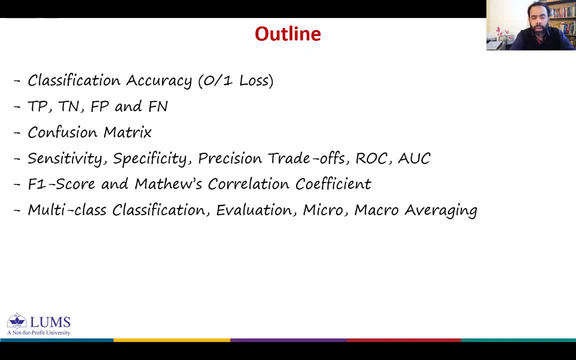 construct a table, what we call confusion matrix or contingency table, and then, from the entries of this matrix, we will define sensitivity, accuracy, accuracy, and then we will define sensitivity, specificity and precision. What are trade-offs between these terms? How can we encounter these trade-offs? How can we study these trade-offs? 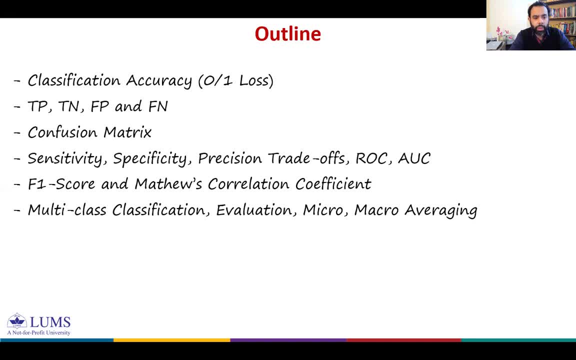 And then we will talk about F1 score and Matthews correlation coefficient. These are two measures to evaluate the performance of classifier. And finally, we will talk about multi-class classification- How to evaluate a multi-class classifier and what do we mean by micro and macro averaging. 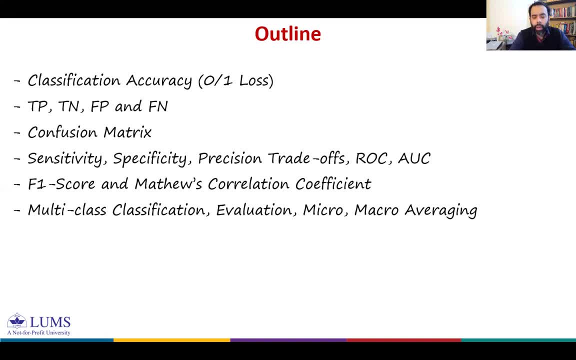 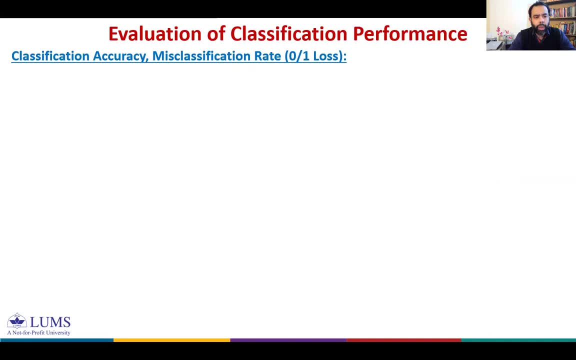 In the context of multi-class classification. Okay, let's start with the classification accuracy. We can define accuracy of a classifier using the zero-one loss function, which we studied in the, I think, the second module, second lecture, in fact. Okay, that's how we defined a zero-one loss function. 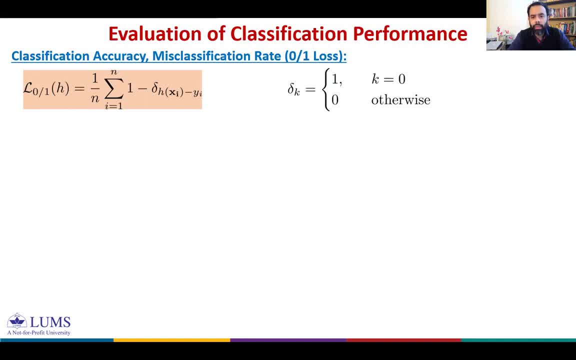 so its interpretation is that for any point x the loss is either zero or one. So this quantity here, which is inside a summation, This quantity can be either zero or one. If the prediction is correct, it means h of xi is equal to yi and delta would be delta subscript zero When subscript is zero. 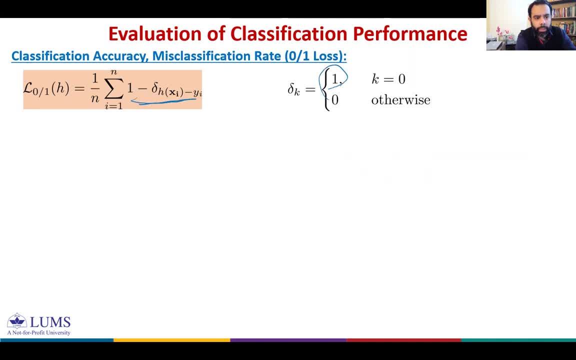 there is a value of one and consequently, this quantity would be zero. When the prediction is correct, it means no loss. When the prediction is incorrect, we call it a loss, Right, so this quantity can be interpreted as the loss. So this term is either: 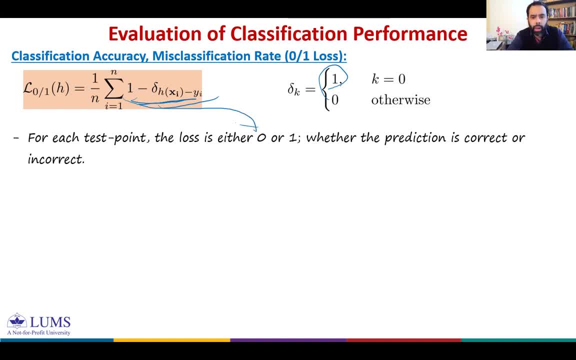 zero or one, It depends whether prediction is correct or incorrect. And when we average over all these n data points we have in the set, So we get this zero-one loss, And this is in fact what we call a multi- sorry, a misclassification rate. Well, this quantity, 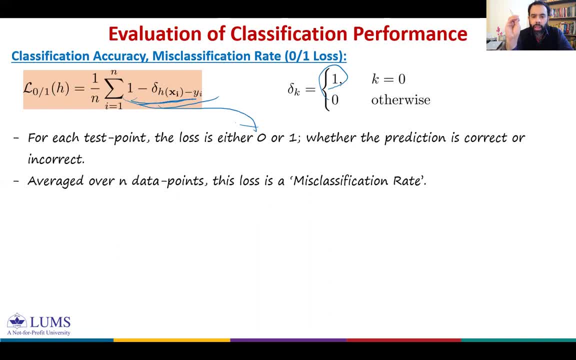 gives the proportion of objects for which classifier is incorrect. for which classifier is wrong, Right, okay, As I said. misclassification rate: estimate of the probability that a point is incorrectly classified. using misclassification rate we can define accuracy, which is simply one minus misclassification rate, right, Or the quantity that gives the proportion of objects. 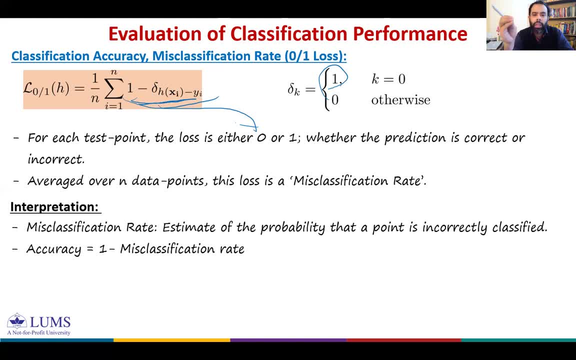 for which the classifier is correct. The classifier is giving you correct predictions, So accuracy quantifies, uh, the amount, the proportion of the data for which the classifier is giving you correct predictions. So accuracy: although it is widely used, it does have some drawbacks, and these drawbacks include: 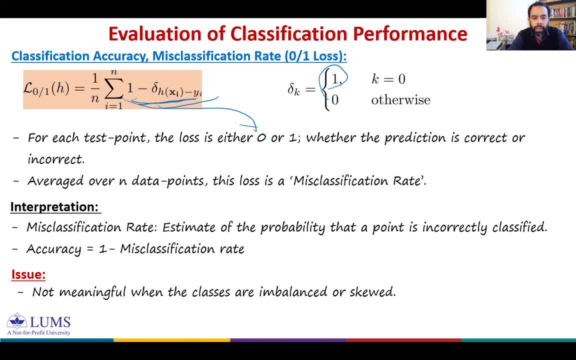 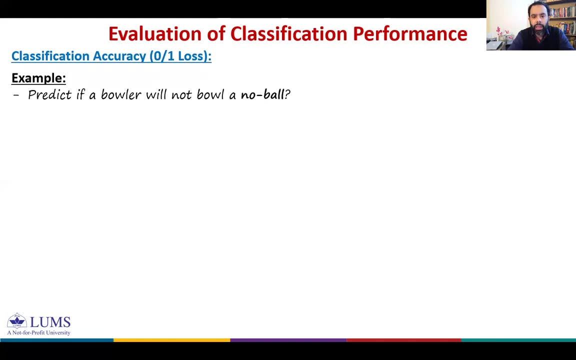 that we cannot use this accuracy measure when the classes are imbalanced or skewed. What do you mean by this? And let me illustrate this with the help of one example. Okay, we take a very simple example that you build a classifier that predicts if a baller 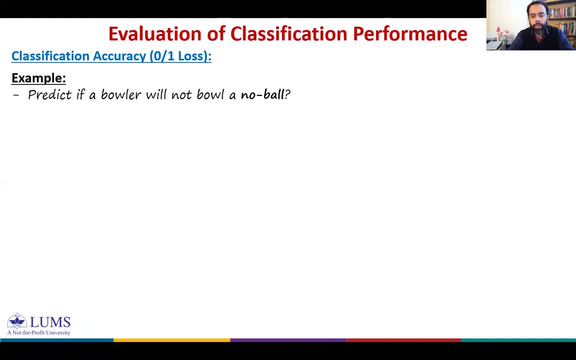 will not ball a no ball. So it's an example from cricket. as we are a cricket-loving nation, We want to build a classifier whether a baller will not ball a no ball. And we assume that in an inning of 50 hours game we have 15 no balls. And if you have a model that says: 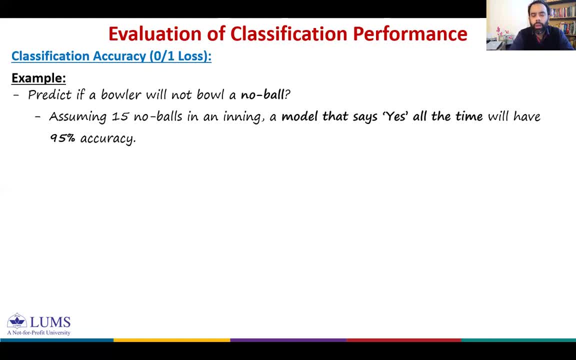 yes, all the time that baller will not ball a no ball. So such a classifier will have 95% accuracy. right, Because the total balls would be 15 plus 300, right, So 50 overs, one over is five balls. 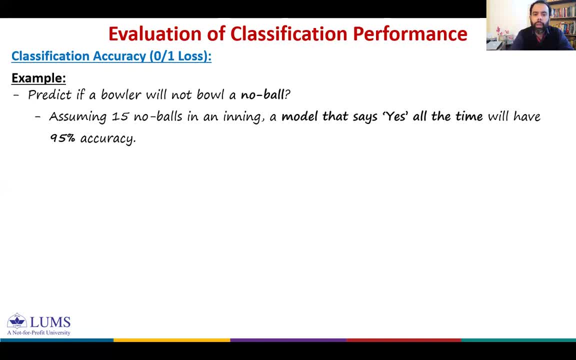 sorry, one over is six balls, three times six, 300, and you have 15 extra balls. because 15 are no balls, You have 315 no balls. A model is saying, yes, all the time that a baller will not ball a no ball. The model would be accurate, in fact 95% accurate, That is. 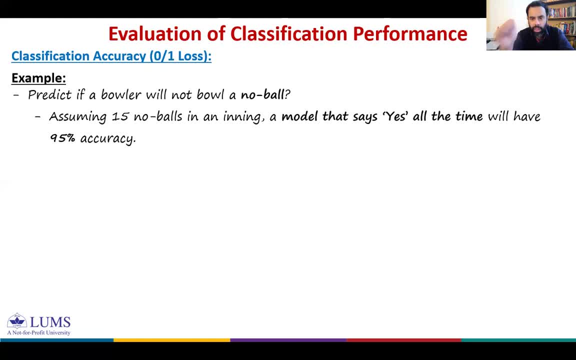 315 times. the classifier is saying: a baller will not ball a no ball, right. So there are only- you know only- 15 misclassifications. Otherwise, the model is working fine, Right? So using this accuracy as a performance metric, we can say that a model is very. 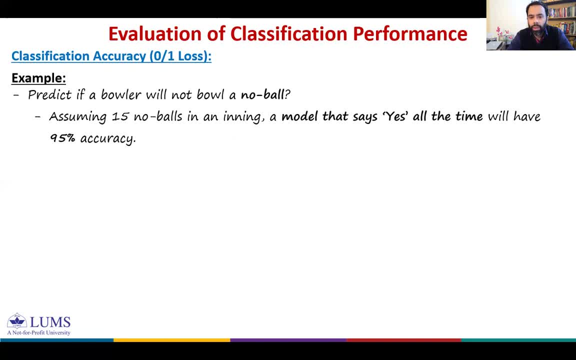 very accurate. But in fact the model is not useful. or model is not valuable, right? Why So total points? we had 315.. We're assuming that there are no other illegal balls, there are no other white balls, And so no ball label, I call it class 0.. And if the ball is not a no ball, I call it class 1.. 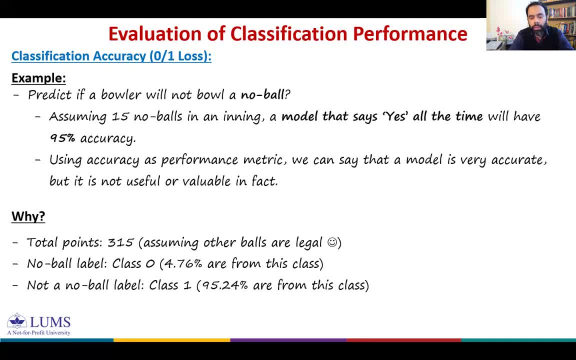 So if you see the total number of balls, or those total number of balls, only 5% balls are from class 0 and remaining 95% are from class one. so we say we have imbalanced classes, right? so in one class we only have 15 elements. 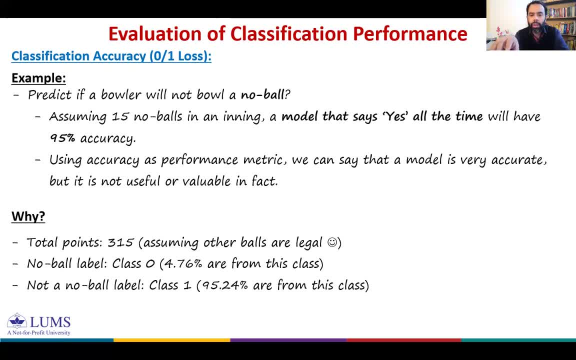 in another class. we only we- have 300 data points. the classes are skewed, the classes are imbalanced and for skewed classes, as we have just seen, it is misleading to use accuracy to evaluate the performance of the classifier right. so this is just one demonstration, one example. 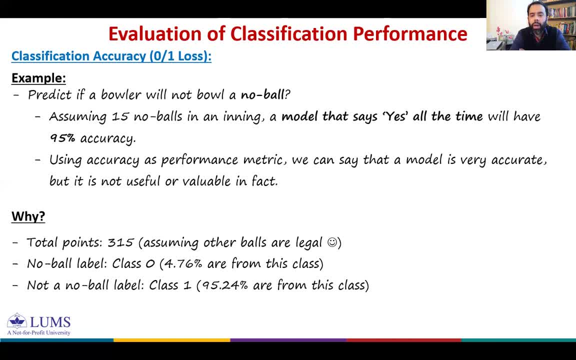 that accuracy is not a good measure to evaluate the performance of the classifier. when the classes are skewed, when classes are imbalanced. in fact, we encounter this imbalancing in all of the applications. for example, we talk about this in the classifier. so in the classifier we are interested in disease detection. 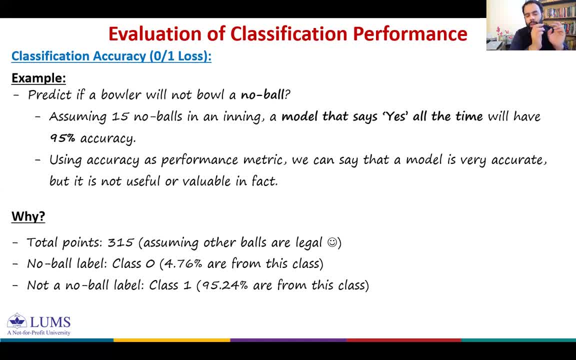 so, given some of the reports of a patient, some pathology reports, some scans, you want to detect whether the person is suffering from a particular disease or not. in most of the cases you would say: you expect the person is healthy, right, and so we have imbalancing in classes. similarly, if you are, 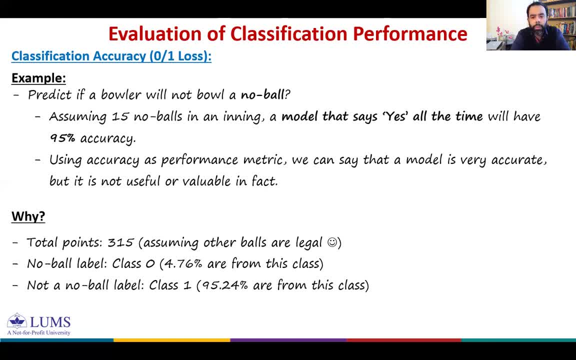 in finance and you want to detect a fraudulent transaction. So you're encountering thousands of transactions every day, but all of those 1000 transactions, only few are fraudulent. So again we have skewed classes. right For skewed classes, accuracy is not a good measure. 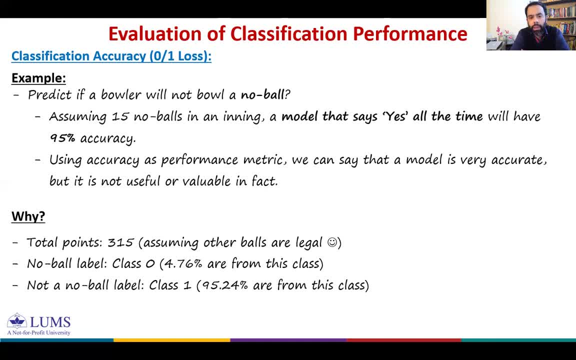 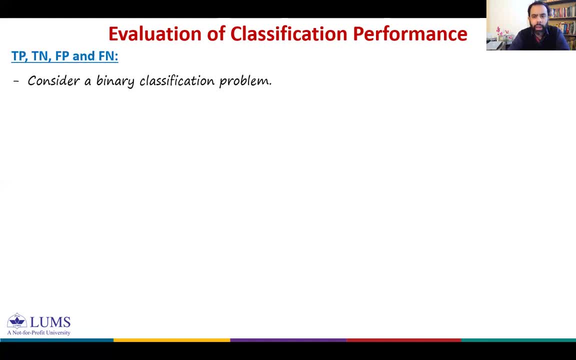 So we need to find out, we need to define some other measures to evaluate the performance of classifier. Okay, to handle this, we'll define the terms true positive, true negative, false positive and false negative, And you often hear these terms when you study the literature of machine learning. 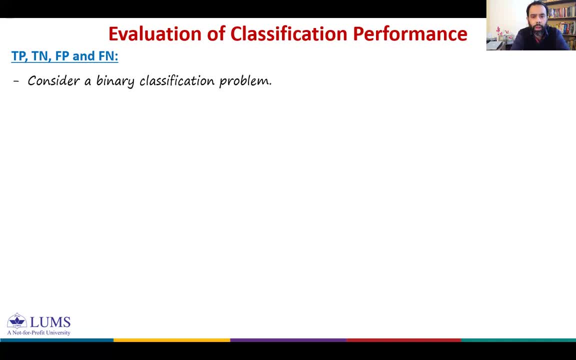 but let's formally define what you mean by these four quantities. To understand these four terms, we consider a binary classification problem, In fact, what we define for a binary classification problem. In a binary classificative problem. we have this dataset. 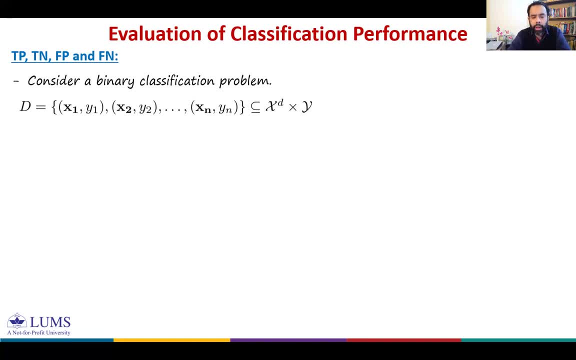 And what about Y? Y can only take value zero or one, right? So we have a binary classificative problem. So set Y would be zero and one. So these are the labels we know right For these: X1,, X2,, Xn. we know the labels for this: X1,, X2, Xn. we know the labels for these: X1,, X2, Xn. we know the labels for these: X1,, X2,, Xn and Y1. 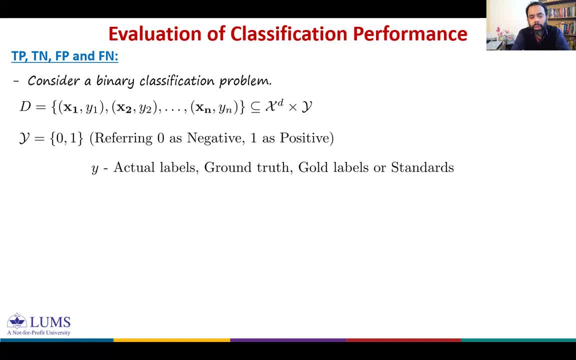 y1,, y2, yn. In fact, if you know the label, we call them actual labels or ground truth, goal labels or goal standards. So these are different terms used in the literature that some you call y as actual label on the data point: ground truth, goal label or a goal standard. 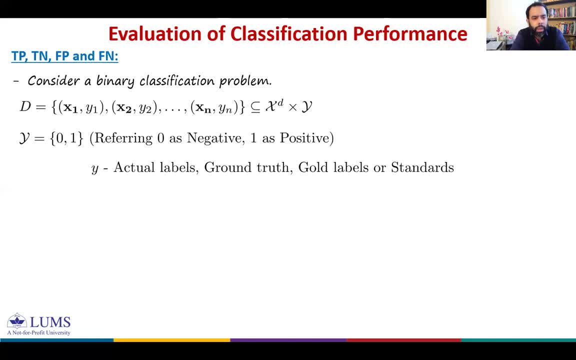 We will refer to 0 as negative and 1 as positive, and this is something very standard. This will help us in defining these terms: true positive, true negative, false positive and false negative. For this binary classification problem, we say we have a classifier h of x. 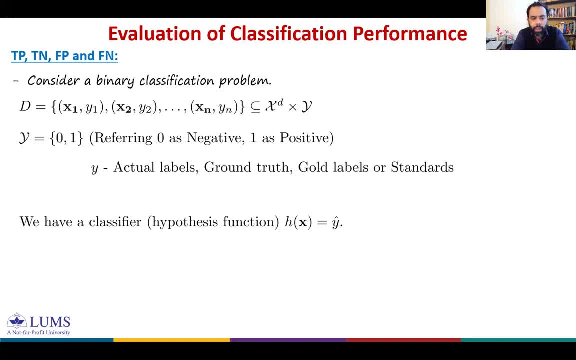 is equal to y hat. So this classifier takes test point from the feature space as an input and gives you an estimate of the label or predicts the label y hat. Again, y hat can be 0 or y hat can be 1.. So both y hat and y can be positive or negative. 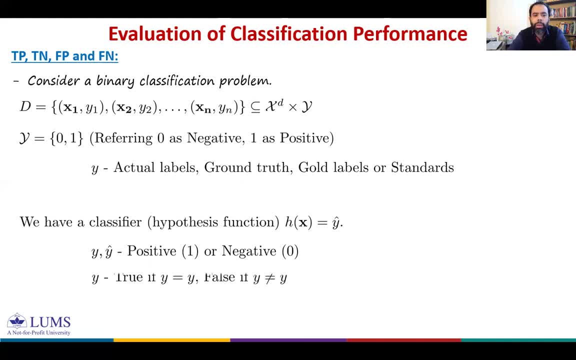 We say y hat as true. if y hat is positive or negative, hat is equal to y, and we say y hat is false if y hat is not equal to y. right, simple. so if you are predicting y correctly, we call it true. if you're not predicting y correctly, we call it false. 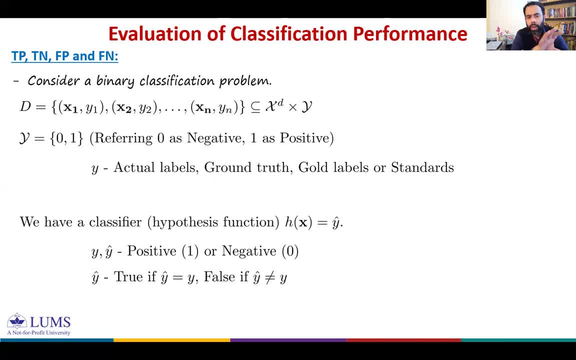 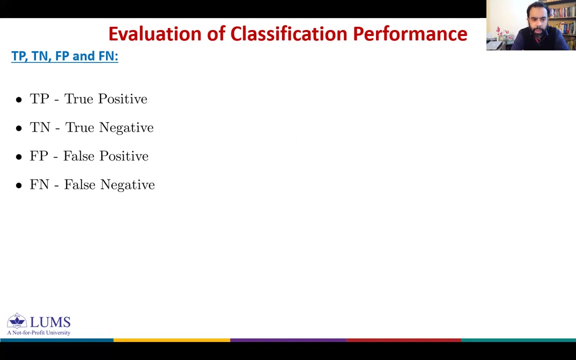 so true refers to correct prediction, false refer to incorrect prediction. positive, positive class one, negative class zero. okay, so, with this understanding, let's move forward and define these terms. okay, we have true, positive, true, negative, false positive, false negative. how do you define true, positive number of points? right, so true and positive, positive means one. 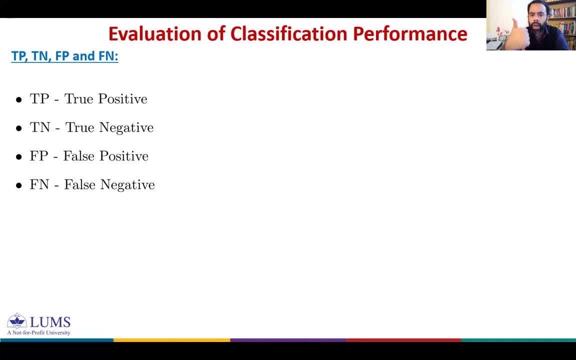 number of points with y is equal to one and your classifier predicted as one: true, positive, true, negative. number of points with goal label: zero, goal label: negative and your classifier also predicted as negative. that's true, true, positive, positive. it is positive in actual. you predict positive, true, negative. it's negative in actual. 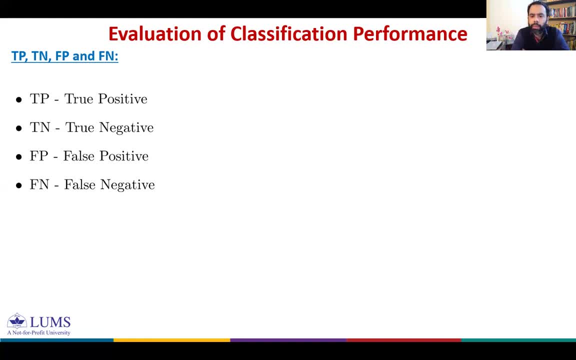 and you predict it as negative. what is false positive? so number of points with y is equal to zero, right, but you predict it as positive. it's false positive. you predict it as positive, but that's the false prediction. similarly false negative. you predict it as negative, but it's a false prediction, in fact. 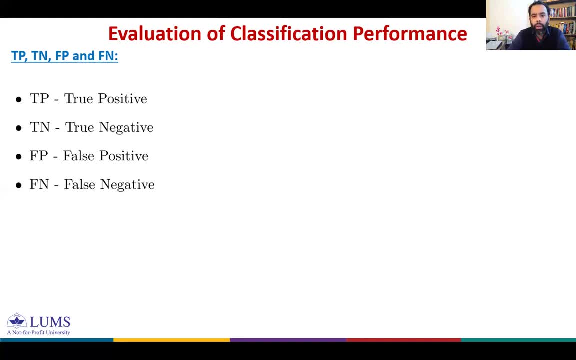 in actual it is, it is one, okay, so yeah. so false negative number of points with y is equal to one, but you classify it as zero. false positive number of points with y is equal to zero and classify it as y hat is equal to one, and so on and so forth. 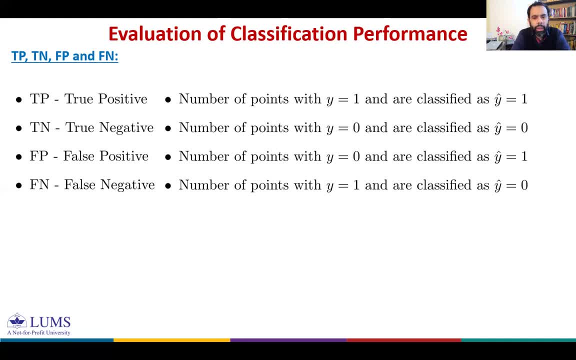 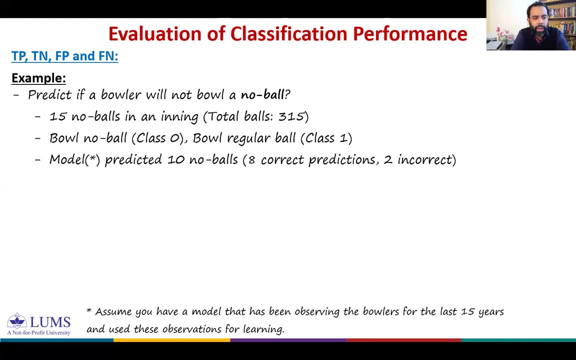 okay, and so let me illustrate, let me explain these four quantities with the help of a couple of examples. okay, again, we take a same example. want to build a classifier that predicts if a baller will not ball a no ball right. so we assume that you have a model that has been. 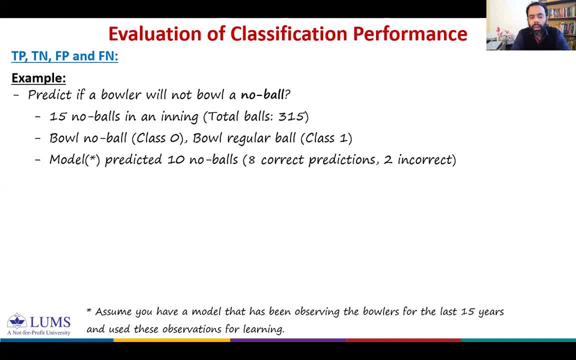 observing the ballers for the last 15 years and use these observations for learning. A baller is going to ball right and you know the current situation. you know the behavior of a baller for the last 15 years and you expect that you can predict that, whether the baller will ball a no ball or not. 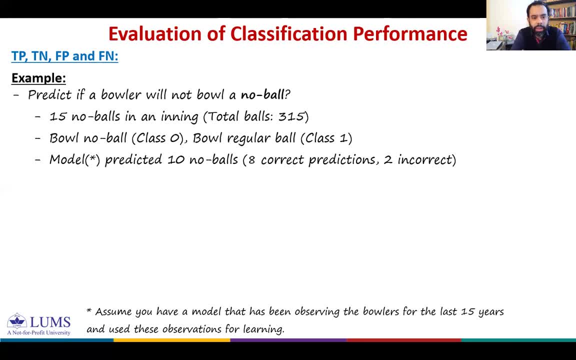 Okay. so if we have 15 no balls in an inning, so we have total 315 balls. As I said earlier, no ball, we call it class zero. A regular ball, or a valid ball, or legal ball, we call it class one. 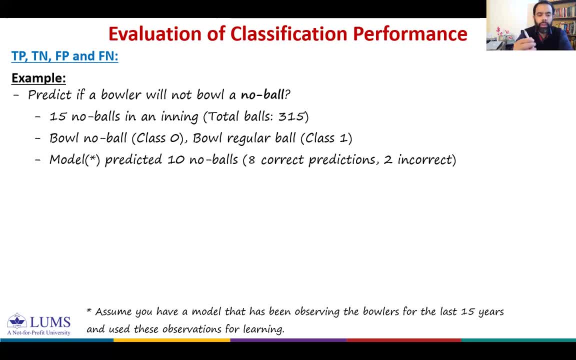 We assume that you have a model that predicted 10 no balls correctly, So we have 10 no balls out of 15 no balls. but when model predicted these 10 balls, eight were correct predictions and two were incorrect predictions. And given this information, we want to calculate true positive, true negative, false positive. 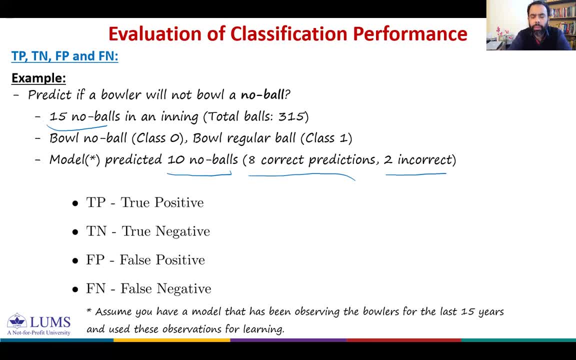 and false negative. Can you help me Comparing this to true? positive means it was a regular ball and your model predicted as a regular ball. So model predicted: two incorrect, no balls. That means so these two are, these two were in fact regular balls. And how many regular balls we? 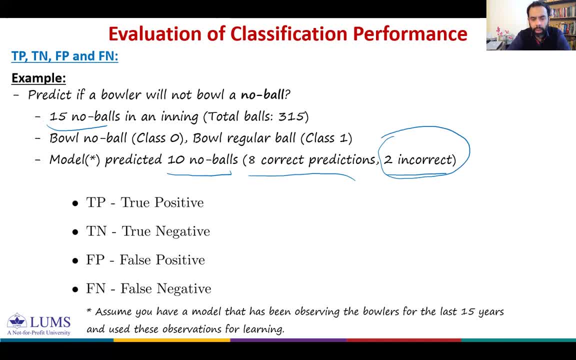 have 300.. Okay, so out of 300, your model predicted two as no balls. incorrectly predicted, That means the remaining 298 balls have been predicted correctly by a classifier, So true positive would be 298.. What about true negative? So negative here: no ball, And you said you could predict eight. 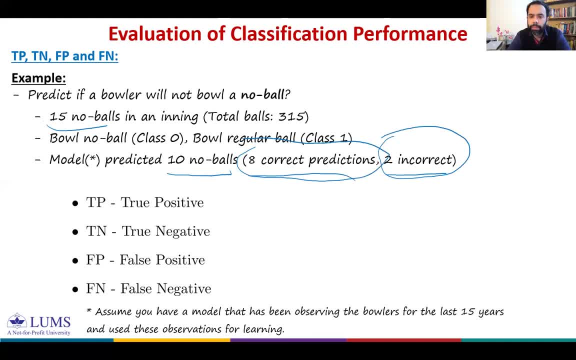 correct: no balls. So true negative is eight. What would false positive? You predicted, as a regular, balls, but they were in fact no balls. So in total we had 15 no balls. You predicted eight correctly, The false positive would be seven. And what about false negative? 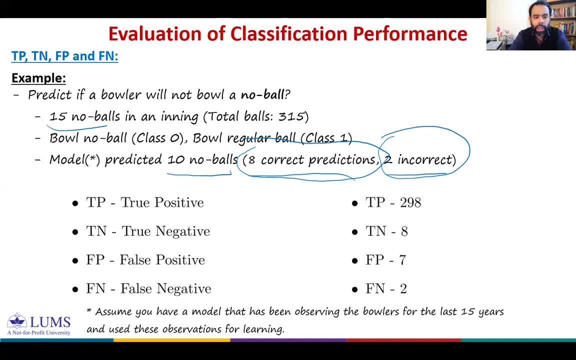 Two. So we have true positive 298, true negative eight, false positive seven and false negative two. I hope this is clear. Okay, so now, using these four quantities, we are going to form a matrix. We will come, we will combine these four quantities and represent in the form of a table. 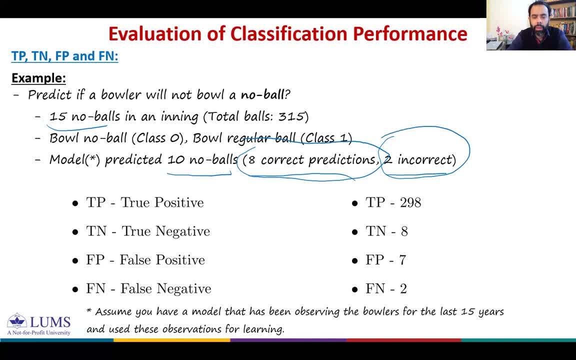 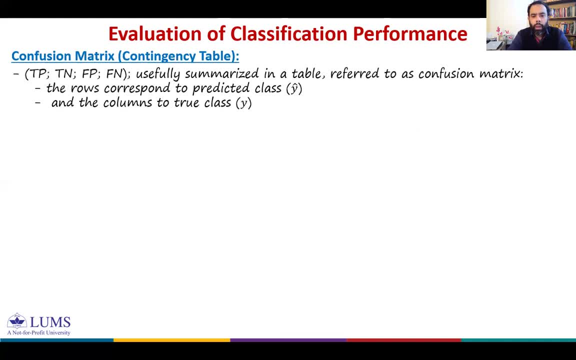 what we call contingency table. In this case, this table will be the generic or common main segment, rather than this common unit table where the numbers are written in. when What that meant was, I was suppose to put two problems first. Second, this return was除ed after a change, because we always 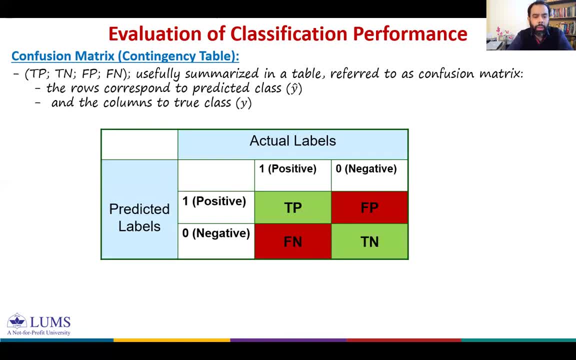 forget how to delete a working table, So this will have the smile. I will say: my student will not delete my table. If she is passive, our table will be as Kw��, and now this is also part of the property of nothing as well. Next we will talk about problems. Give me an example. 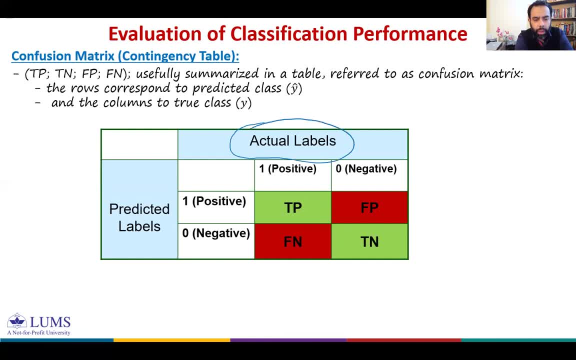 So let me talk about a cone matrix. Okay, I can see a cone matrix, All right, let us see A cone matrix. Let us talk about the green matrix. Let us talk about confusion matrix. Okay, So that's how a cone matrix looks like. Let me explain this. 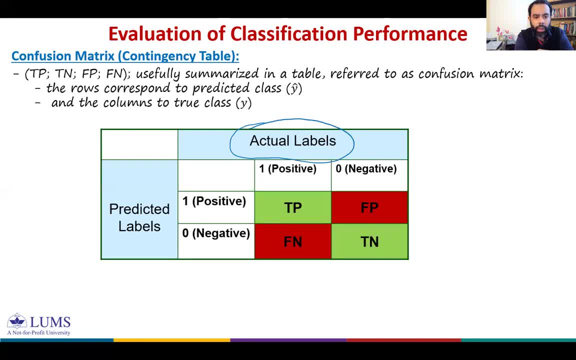 gold standards and XT label can be positive, XT label can be negative. predicted label can be positive or negative. so the quantity here, this is true, positive. that means the actual label is positive and you predict it as positive, false positive. you predicted positive, but there's a false prediction. 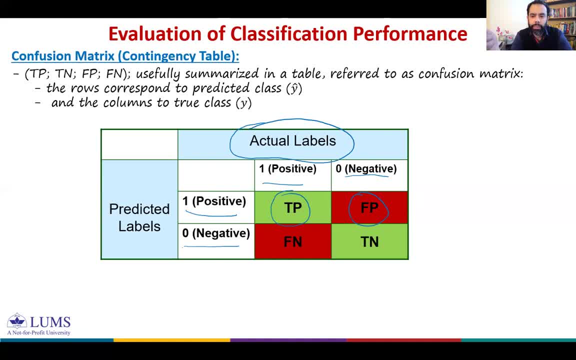 actually so those points were negative. F, false negative. the number of points with actual label positive, but you predicted as negative, so N indicates okay, this second is what you predicted and the first F is, if it's a false prediction as a true prediction, similar to negative, what's the? 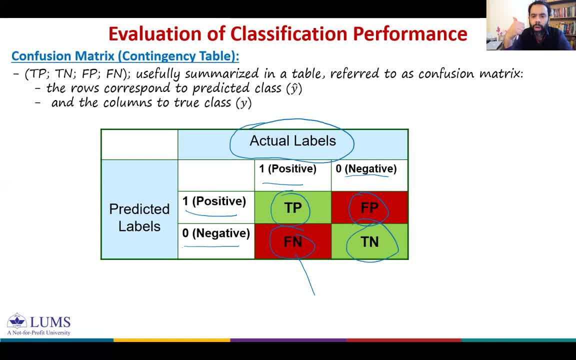 interpretation. number of points with Y is equal to zero and you also predicted Y hat zero, right. true, negative. okay, if we should sum these two terms- tp and fp- true positives and false positives- so what you get is a total number that model predicted as positives. similarly, if you 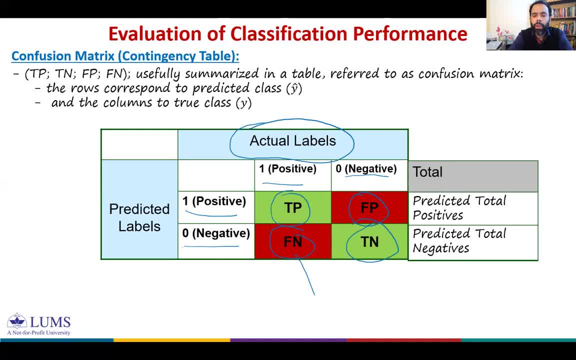 add false negative to negative, you get total negatives, the model predicted, and if you sum along each column what you get is actual total positives and actual total positives- negatives. so p denotes the actual total positives in your data, the number of positives or the number of points in your data set with one as goal level and number of points in your data set with zero as 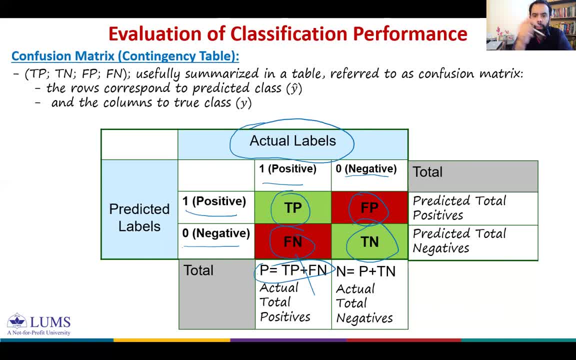 goal level. okay, i hope this is clear, right? so now, if you see a confusion matrix and you see these terms- true positive, true negative, false positive positive- uh, you should be able to clearly interpret the results in the table or the information given in the table. okay, let's, let's learn further, and let me illustrate this with the help of a couple. 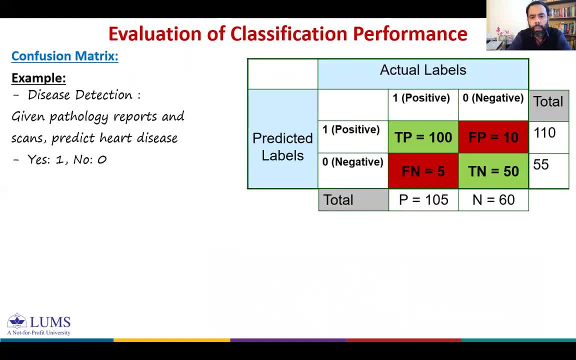 of examples. okay, we take example from disease detection. so, given pathology reports and scans of a patient, we want to predict. your classifier predicts whether the person is suffering from heart disease or not. so if the heart disease is detected, you call it. yes, this means positive class, no, zero, negative. 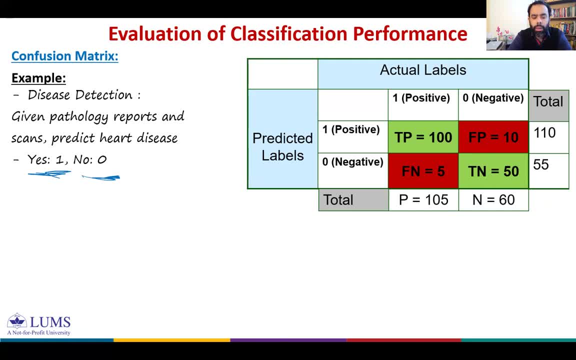 class, okay, and uh, you carry out analysis on 165 patients and you find true positives to negative, false positive, false negative, and you construct this confusion matrix given. okay, if you're given this confusion matrix, how would you interpret this confusion matrix? what is the interpretation of this confusion matrix? okay, first of all, you would say that p is always positive and you: 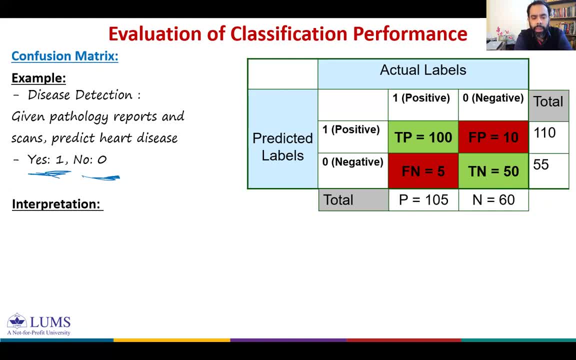 would say that p is 105 and is 60. so in total we had 105 plus 60, 165 patients. we had 165 cases, we had 165 data points. so out of those 165 data points- right, so we had 105 with. 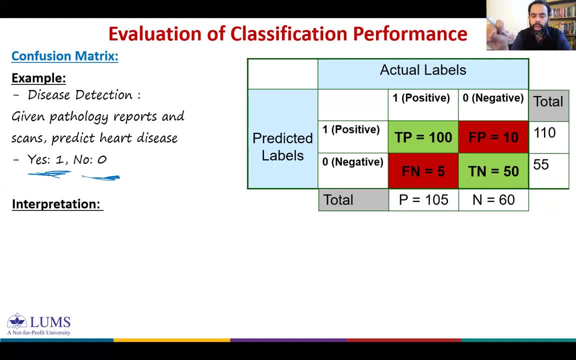 a positive label and 60 with negative label. so we had 105 cases with heart disease and 60 cases of healthy patients. of healthy people, in fact, it's not a patient, okay, and uh, how do you interpret true, positive? so out of those 105 that were that were labeled as, uh, diseased patients. so your model could predict. 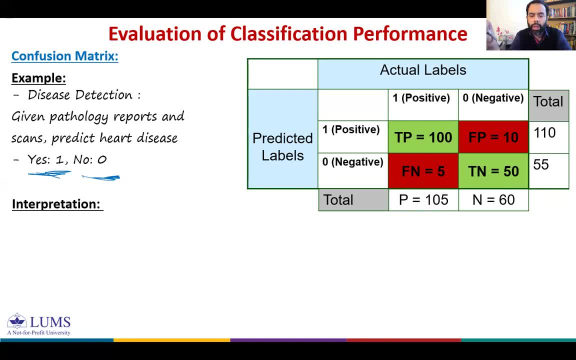 100 as disease patients, but your model could not predict five out of those 105 as visible. so you say your model predicted yes 100 times and no 55 times. so in reality, uh, yes as 105 times and no is 60 times. sorry, hang on, it should be. 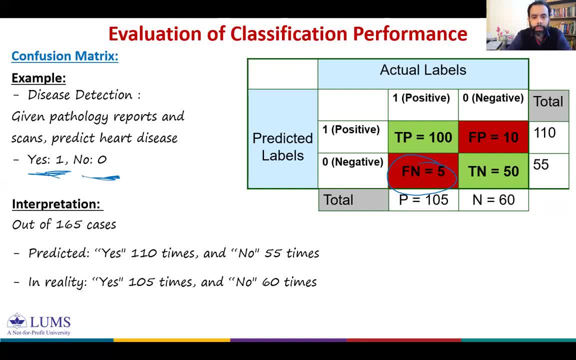 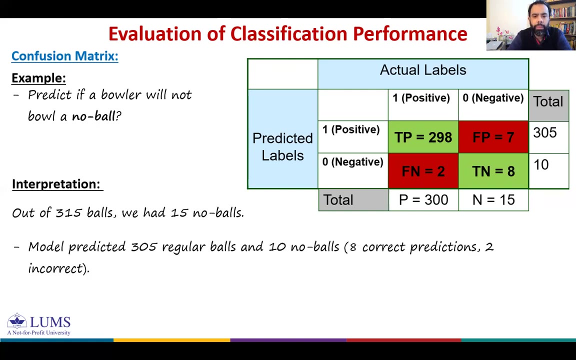 yeah, it's all good, okay, uh, i hope this is clear. let me give you one more example. we go back to this. that's no ball balling example. we use same information and i construct this contingency table interpretation. so your model predicted 305 regular balls. this is zero five. 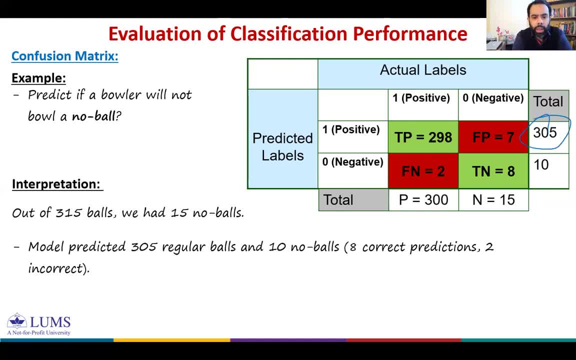 okay and 10 no balls. and out of these 10, the two were incorrect predictions and rv 305. seven were incorrect predictions and if you see a long column out of 300 regular balls, your model could predict 298 regular balls. and out of 15 no balls- 15 in the zero class- your model could predict eight no balls correctly. 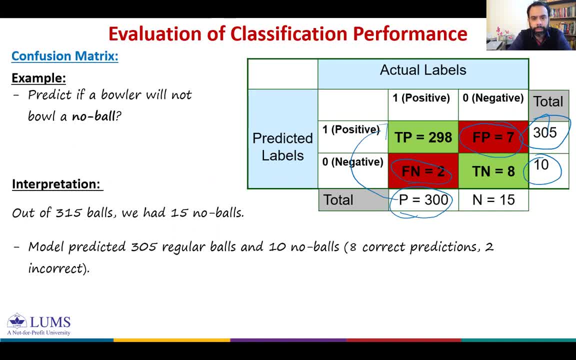 okay, i think this is clear now. okay, now we have a good, good understanding of confusion matrix, i am going to define some of the matrix, some of the measures, using confusion matrix. so we know true positive, true negative, false positive, false negative. using these four quantities, we will define some measures to evaluate performance of classifier. 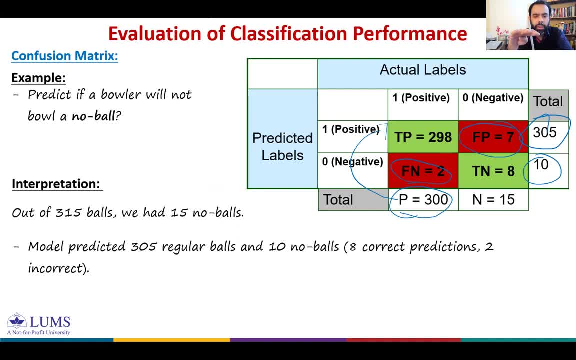 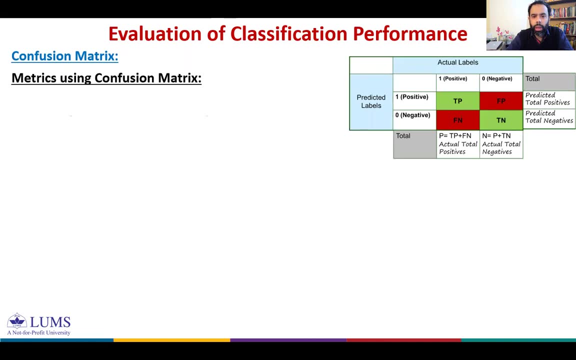 so these four- true positive, true negative, false positive, negative, these are not measures, right? so these are the just some quantities coming from the output of a classifier and we will use these quantities to define some layers. okay, uh, we start with, uh again, accuracy, if i ask you, uh, that one zero loss accuracy, um, so one minus misclassification rate. 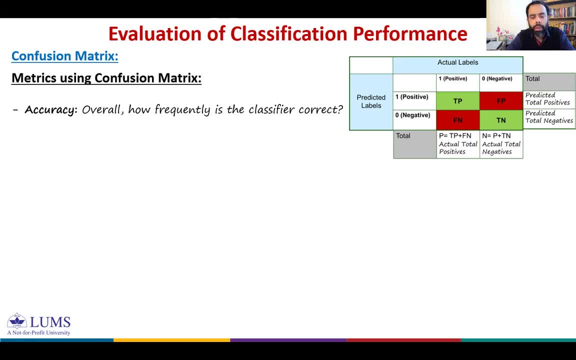 if you want to find the same accuracy using your confusion matrix, can you find out? in fact you can. so accuracy would be true positive plus two negative plus two negative divided by total number of points. true, positive indicates the number of points. number of positive points your model predicted as positive. true, negative number of points in class zero. 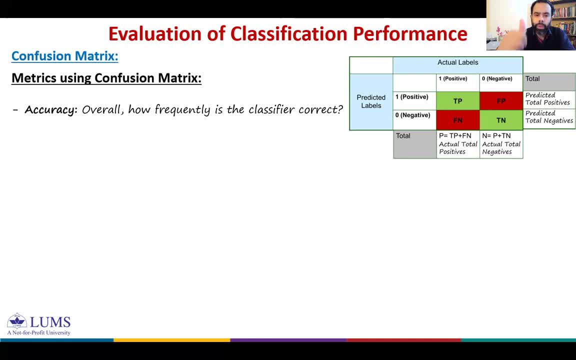 which your model could predict in class zero. so true positive plus two negative divided by sum of these four. so what you get is accuracy. so mathematically we say that accuracy would be given by true positive plus two negative divided by total number of points you have. 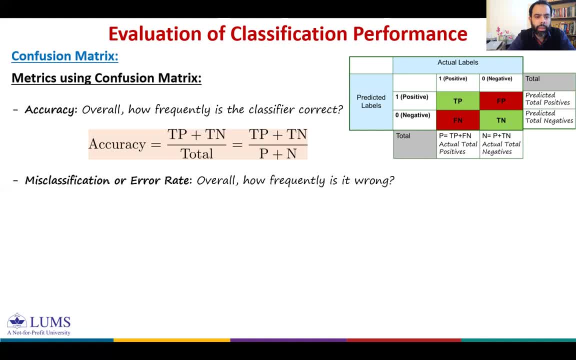 uh, okay. misclassification or error rate: uh, overall, how frequently it is wrong? mathematically it is given by false positive plus- hang on, uh, plus false negative divided by total number of points. or this is just one example, this is just one- minus accuracy, okay, so these are very obvious terms. let's define some, uh, some good measures. 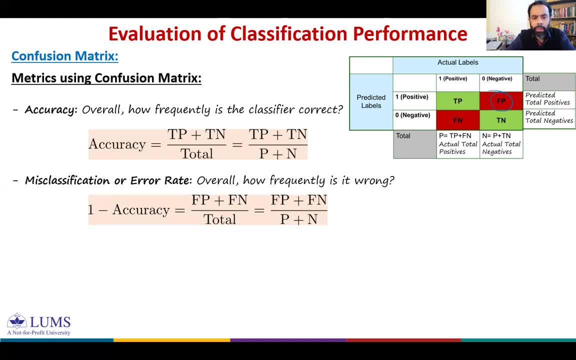 or some practical measures. the first one is sensitivity. we also call it recall, and there is a reason why we call it recall. i will explain shortly. and true, positive rate. so how often does your model predict positive when it is actually positive? if i give you this concrete matrix and i ask you to compute this proportion, 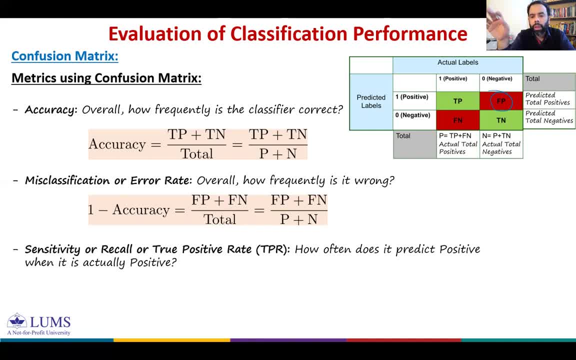 right. so we want to find out out of all the positive data points, all the data points that are that had the goal label, how many have been truly identified as positive by our classifier? and so we get this: what are total number of points with one as gold label, t, p plus f n p right and out of these p? 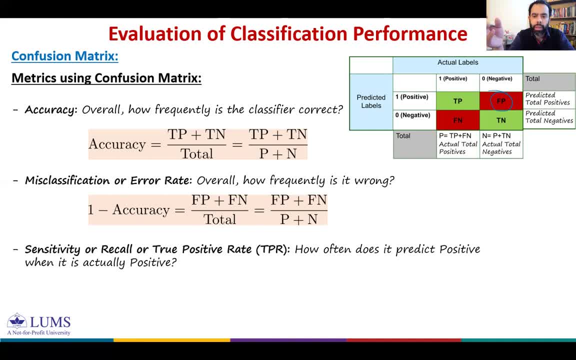 points, you could predict t p points. so a true positive rate of sensitivity or recall is given by simply true positive right, where true positive is false negative right. in case you forget, this is true positive right and we're going to start to run our model and see what's going on with this model. 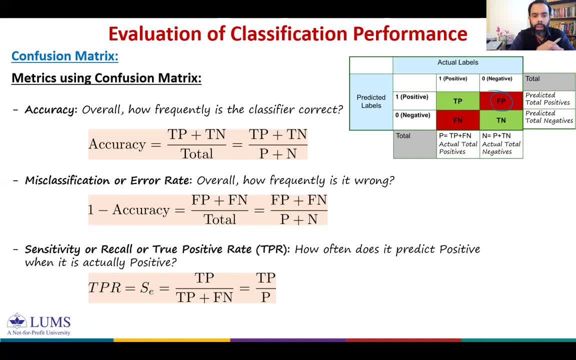 forget this formula. You don't need to. in fact, you don't need to remember this. You simply look at the table and you take true positive rate. you take true positive and you sum along that column and you get a recall, or sensitivity, or true positive rate. TPR is simply TP divided by the. 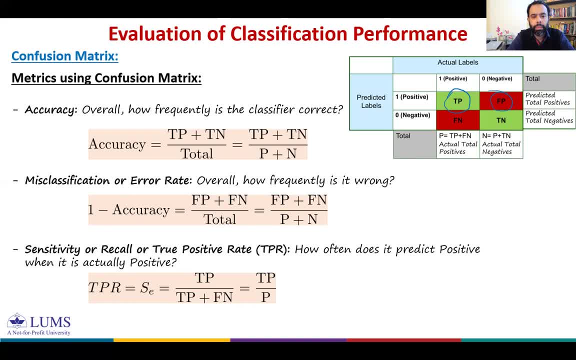 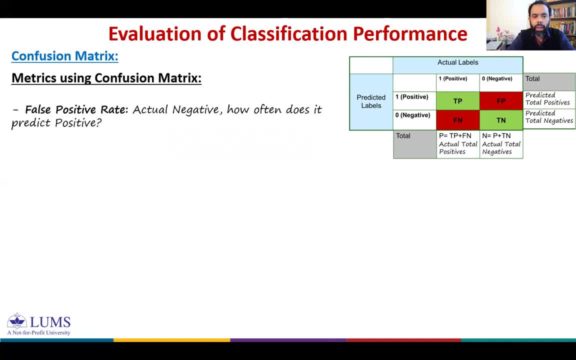 values of the column in which TP is present. Right, Simple, Let's also define some more metrics. False positive rate, as the name suggests. So actual negative. how often does it predict positive? It's a false positive rate? Okay, Okay, I think now you're trained. 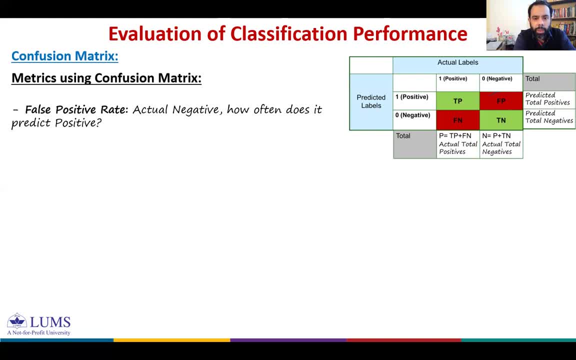 enough That you can compute this. It will be simply given by false positive divided by the number of points. So all the points in the column containing false positive Or FPR is given by false positive right By total number of points with a label of negative class. 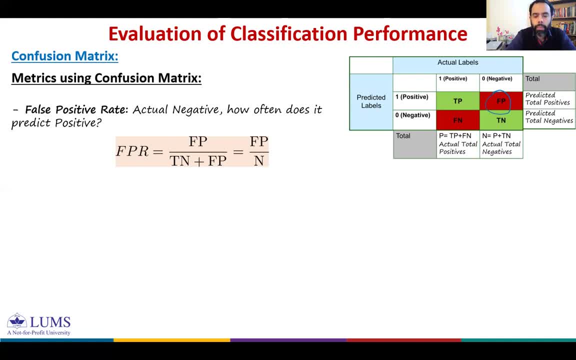 label of class zero. Okay, Okay, Let's talk about, let's talk about, let's talk about another metric: specificity. specificity or true negative rate. When it is actually negative, how often does it predict positive? So actual label is negative and you predict. 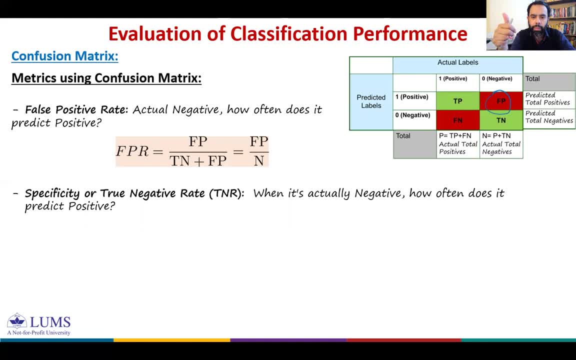 as positive, Right? Where do you get it? Hang on, So it's a true negative rate when it's actually negative. And how often does it predict It should be? my apologies, It should be. I will correct this in the notes. 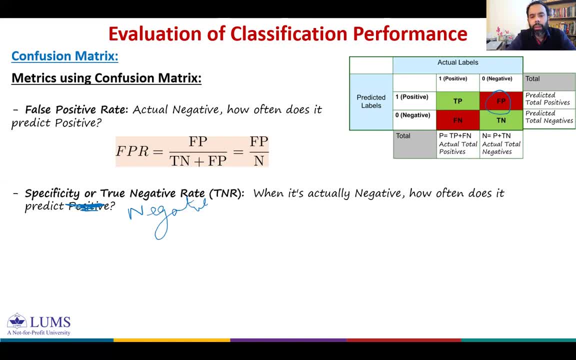 Negative. So true, negative divided by N, And there is simply one minus false positive rate. Let's define some another metric which is very, very important. So true, negative divided by N. Okay, So true, negative divided by N, And there is simply one minus false. positive rate. Let's define some another metric which is very, very important. So true, negative divided by N, And there is simply one minus false positive rate. Let's define some another metric which is very, very important, What we call precision When. 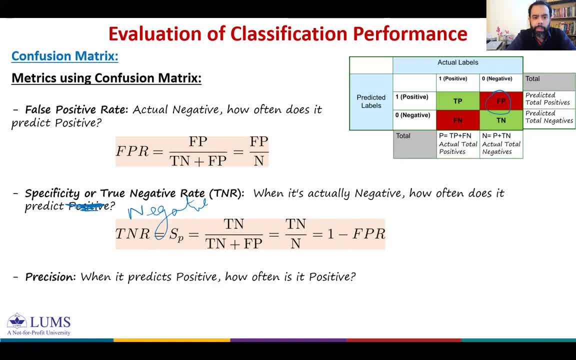 it predicts positive. how often is it positive? What do we mean by this? You predicted as positive and out of those positive predictions, So how often is it positive? How many points out of the total positive points had goal level as positive? That was simply given by. if you 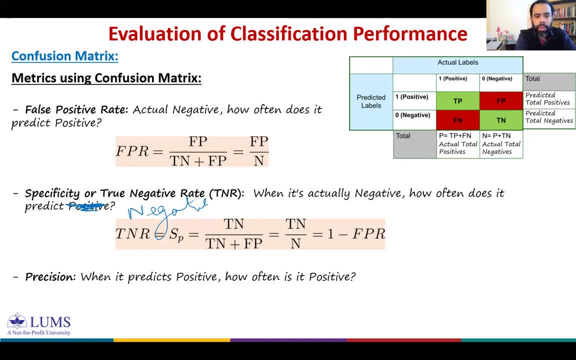 see in the matrix table you sum TP and FP, you get total positives predicted right And out of these total only TP had TP is capturing TP and N is saying that this is positive number of points had the actual positive label. So precision would be given by simply. 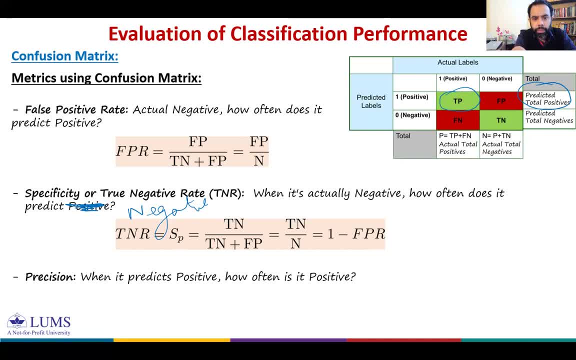 a ratio of Tp divided by predatory rotor positive, that is, Tp plus Fp. So that's how we define precision. I hope this is clear now. So sensitivity, specificity and precision, And we will study these terms in detail. So what is precision When it predicts positive? 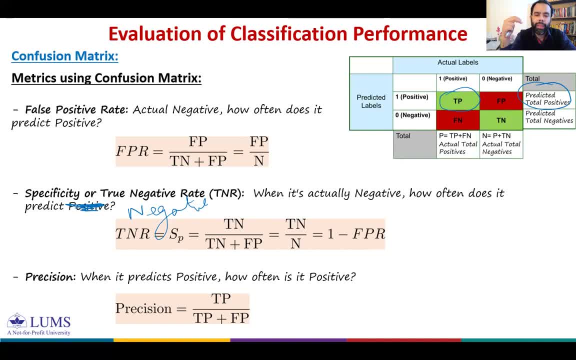 how often is it positive? Sensitivity? So what was sensitivity? Tp over Tp plus Fp? When it is actually positive, how often does it predict positive? Okay, let's move forward, And let me summarize all of this from the confusion matrix. 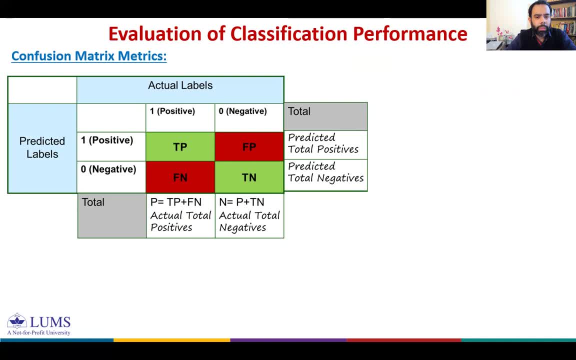 So we have this confusion, matrix. And what is sensitivity? True positive rate, So Tp divided by sum of all the terms in this column, Tp over Tp plus Fn. If you use the second column and you use true negative rate by ratio, you get true negative rate, which is also called 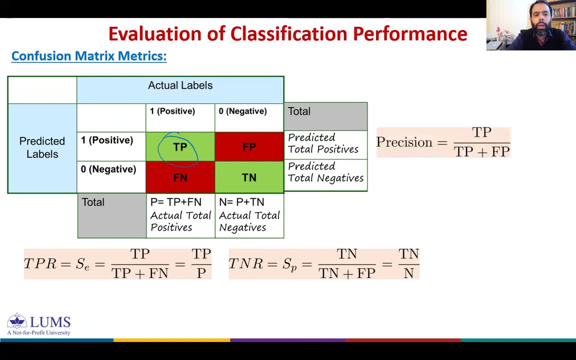 specificity. So we have precision, which is simply true positive divided by a sum of these two. We have theва, which is now a measured complexity, L brabh, by the sum of all the details in this column And this quant. it is given by true negative divided by true negative plus false negative. 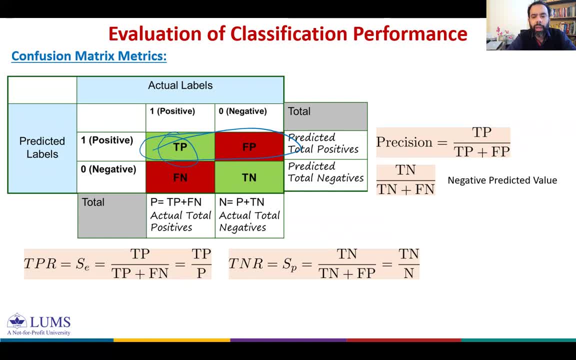 Okay, that is when it is negative. how often does the model detect it negative? Let's use productivity to predictお願い negative values which are negative, and I, hitting negative, predicted your total negative values, which are Tn plus Fn, and you divide Tn by this quantity. 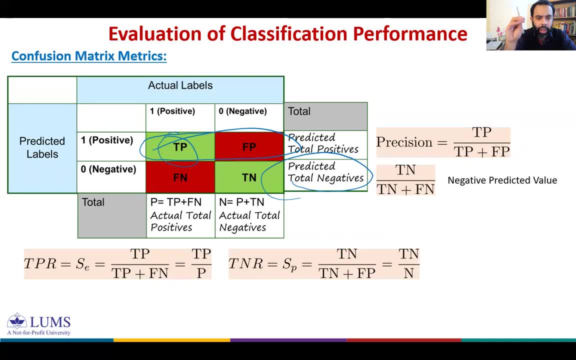 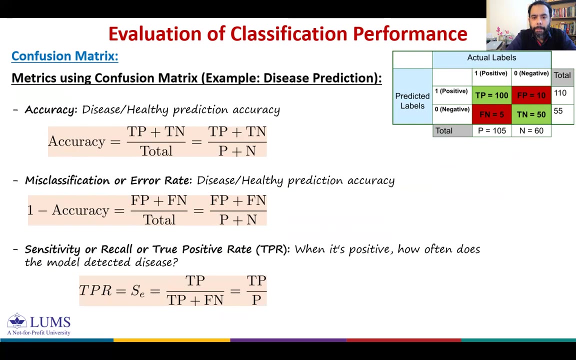 That means, out of total predicted negative values, how many values had the label zero? had the label negative? Okay, let's compute these terms for the disease prediction example. Okay, we had this confusion matrix for disease prediction example and we want to compute accuracy, misclassification rate, sensitivity, true negative rate and precision. 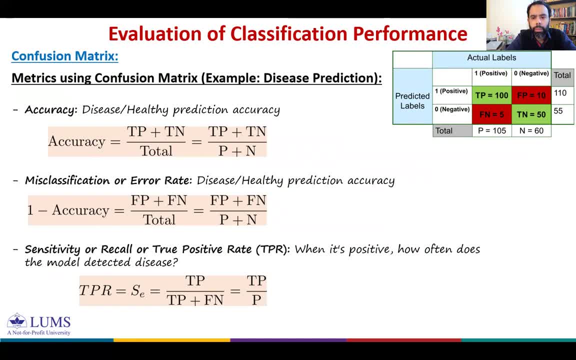 Okay, accuracy: how would you compute it? Total patients: 165, true positive: 100, true negative: 50.. So accuracy should be given by 100 plus 50 divided by 165.. 0.91, right Misclassification rate, now one minus accuracy: 0.09.. Sensitivity or recall: how would you compute sensitivity? 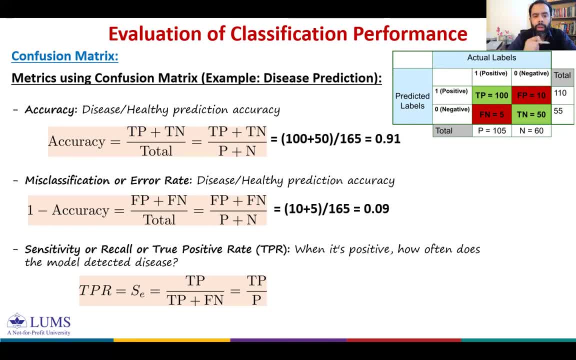 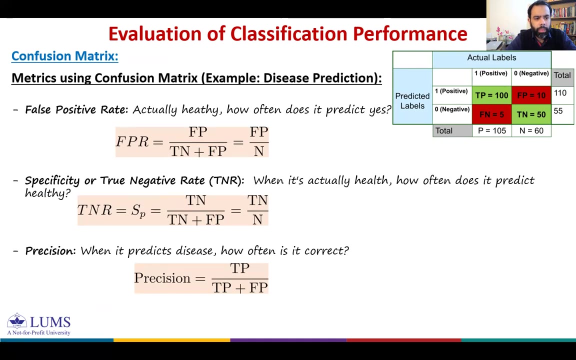 And what is the interpretation of sensitivity When it is positive and the person when you have a disease patient, how often does the classifier detect a disease? Okay, that is 100 by 105, that is 0.95.. Okay, false positive rate, so actually healthy. but your model predicted healthy. 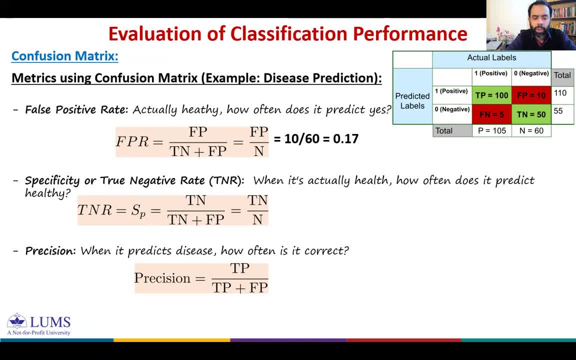 That is simply false positive by n. that is 10 over 60.17.. Sorry, actually healthy. how often does it predict diseased? That is 10 over 60? because it's false positive rate Your model predicted as positive, but there's a. 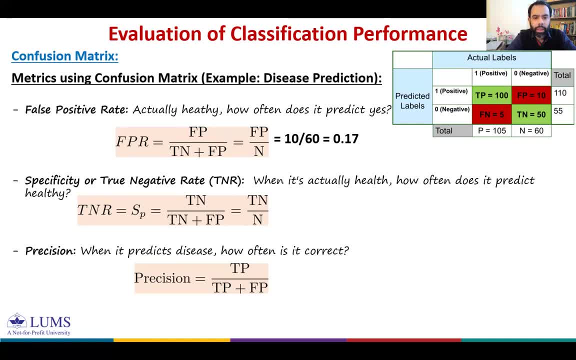 false prediction. In fact it is. it has a negative label: TNR specificity 50 over 60- that is 0.83, and TNR specificity 50 or 60- that is 0.83, and tnR specificity 50 over 60.3. and tnR the disease. 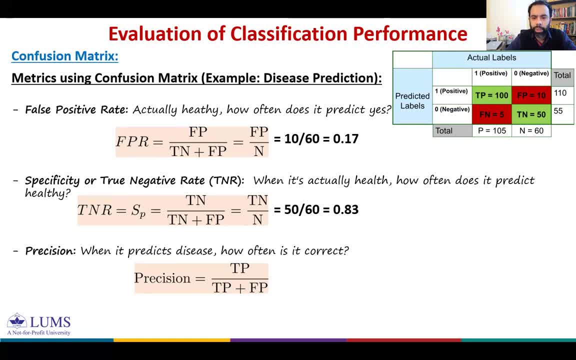 and precision would be simply- you can compute it- 100 over 110.91. but you need to look at the interpretation of precision. The model predicts diseased patient. how often is it correct? because you don't want all the patients to be incorrectly classified as diseased. so precision is important in disease prediction. 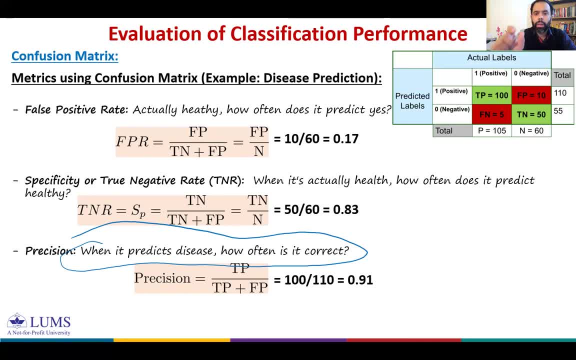 you want to precisely classify patients as diseased or healthy. okay, we have defined too many metrics, right? but I think we will keep on using these metrics and and you will be comfortable with with these. the question here is, out of these metrics, when to use and which one to use. 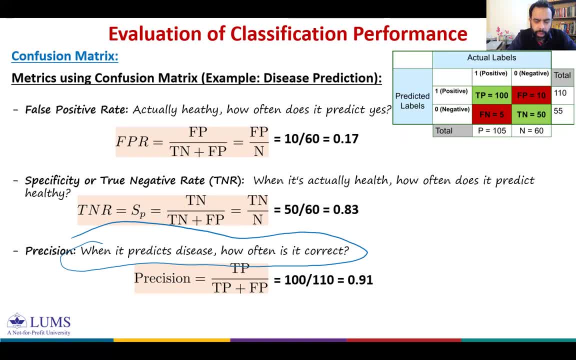 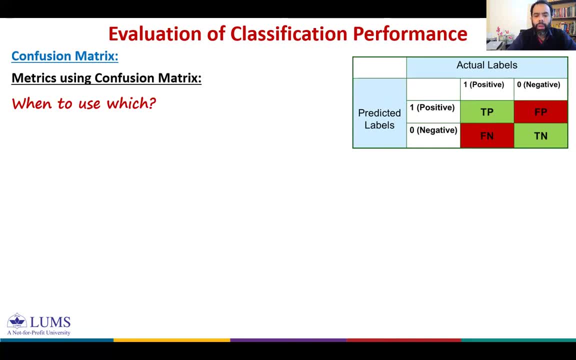 to evaluate the performance of a classifier? right? to answer this question, maybe we start with a couple of examples. so again, consider our disease detection problem. right. in this problem we do not want to have false negatives. so we should take the metric out of all the metrics which have a false negative in the denominator and our model should give higher values for that metric. 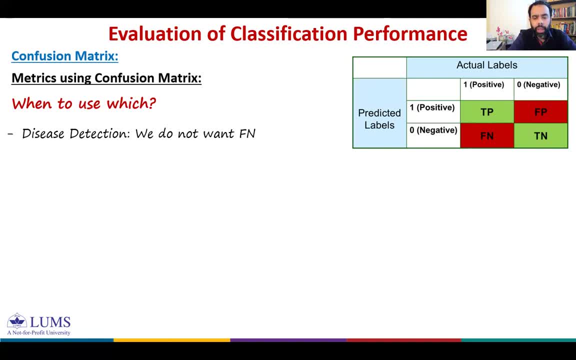 if you go back and see all the metrics, which of the metrics had a false negative in the in the say, say the denominator. So if you recall the true positive rate, so had FN in the denominator, so true positive rate sensitivity recall If you want to lower FN. 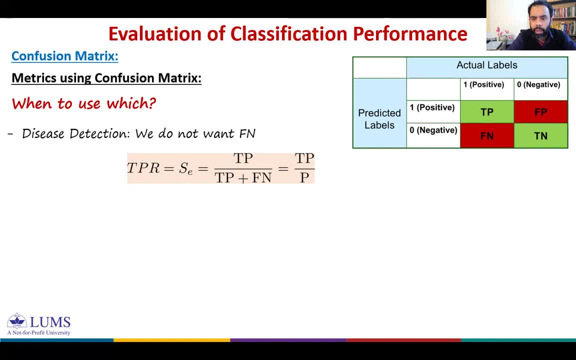 if you want to have less number of false negatives, you should be having high value of should you would require. you would desire the TPR to have high value, okay, So what about this example? In fraud detection, you do not want false positive right. 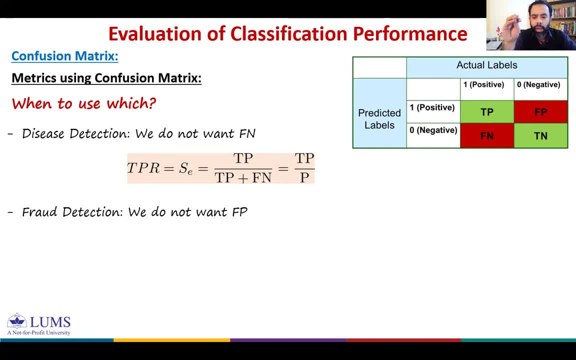 So I'm assuming that fraud is considered as positive and not fraud is negative. So we need to be absolutely sure when we say it is fraud. we cannot afford to have false positives in fact right And when we want false, when we do not want false positive. 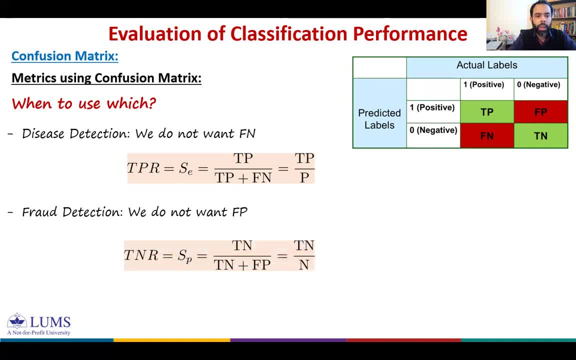 or we want false positive to go produce. we can use true negative rate as our metric, because in true negative rate we have false positive in the denominator. Hard value of true negative rate implies low value of false positive right. Or instead of TNR, you could also use precision. 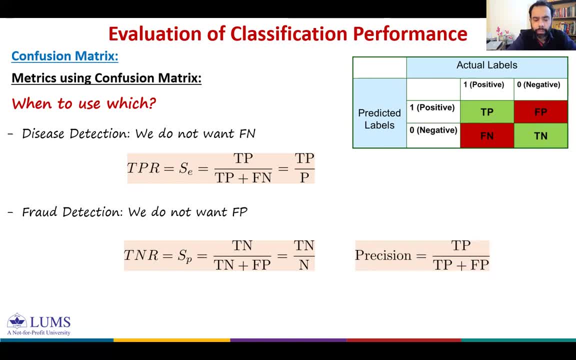 because in precision, we also have false positive in the denominator Okay. Okay, so we conclude this video. We have talked about the issues with the accuracy as a measure to evaluate performance of a classifier. when we have imbalanced classes, when we have skewed classes, we should not use accuracy as a 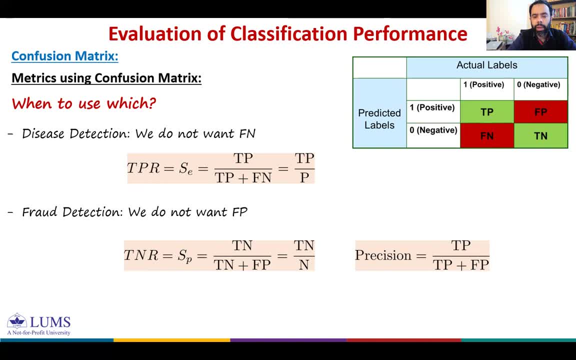 measure. and then we defined true positive, true negative, false positive, false negative. using these terms, we construct a confusion matrix. and from the confusion matrix, from these, using these four quantities, we defined a couple of new metrics to evaluate the performance of classifier. okay, we will stop here, and in the next video i will talk about the trade-off between these metrics. 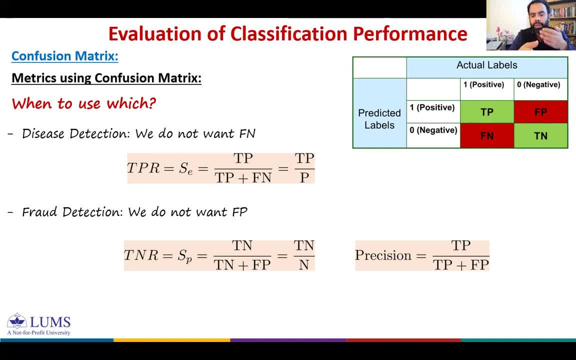 especially the trade-off between precision and recall, precision and sensitivity, and sensitivity and specificity, and how do we study, how do we analyze questions, these trade-offs? Okay, I'm gonna stop here and see you in the next video, inshallah.